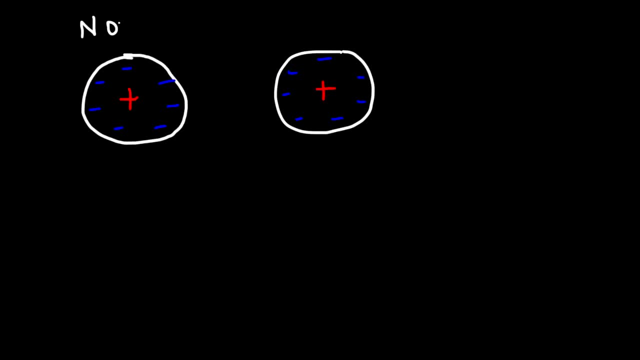 are evenly distributed in an atom. you're going to have a nonpolar atom Now, because the electrons are constantly moving. there's going to be times where one side of the atom will have more electrons than the other side. In this case, the electron cloud is now distorted. 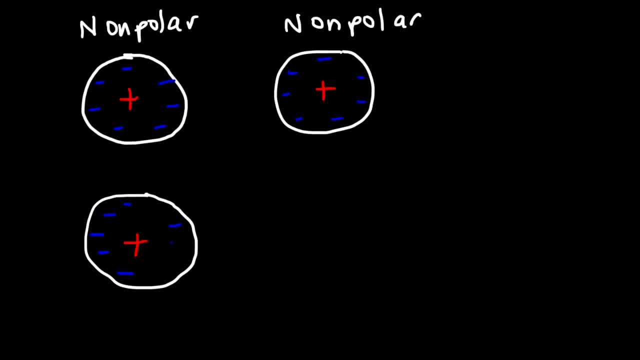 So we have an excess of negative charge on the left and a deficiency of negative charge on the right side. So basically we could say that this particular picture now looks like this: So there's a net negative charge on the left and because the right side is, 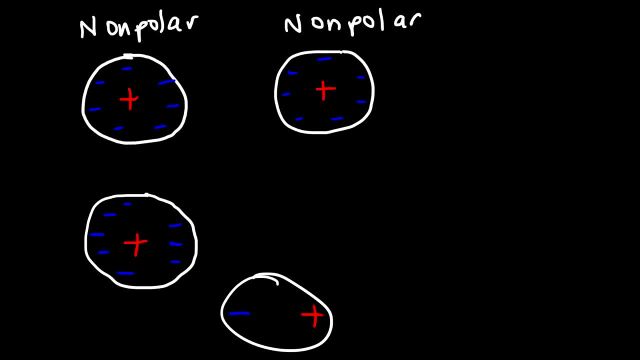 electron deficient, it's more positively charged now. Now, granted, there's still negative charge on the right side, but this positive charge means that it's less negative than the left side. So now this atom is now polarized, It's now a dipole. Now this dipole doesn't last long, So it may last for a 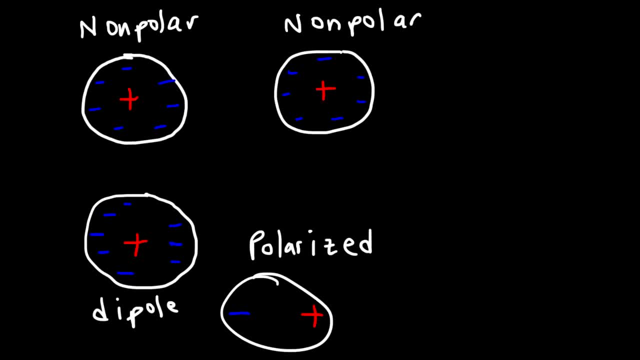 very, very, very short time. So it's a temporary dipole. What happens if we take this dipole and place it next to a nonpolar atom where the electron cloud is evenly distributed, The electrons will flow force that will accelerate them Towards the positive side of that atom, And so this electron cloud becomes. 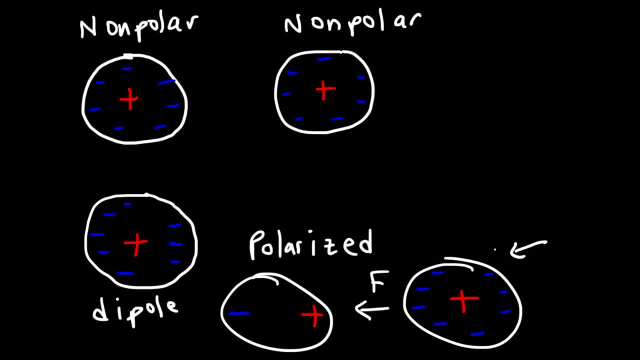 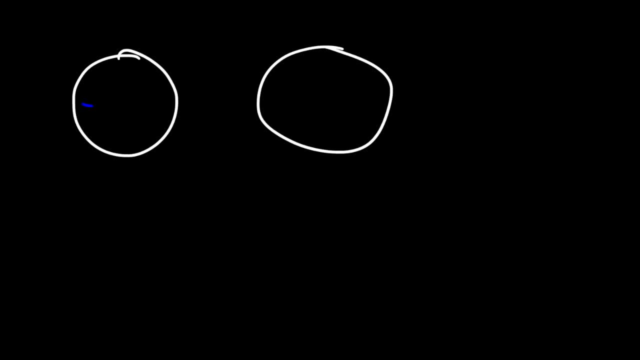 distorted, And so this atom becomes polarized. And so what happens is now you have two polarized atoms. Now you need to be familiar with a term called polarizability, And it basically describes the probability of the atom being polarized. So let's compare fluorine and iodine. Fluorine has nine electrons, Iodine has 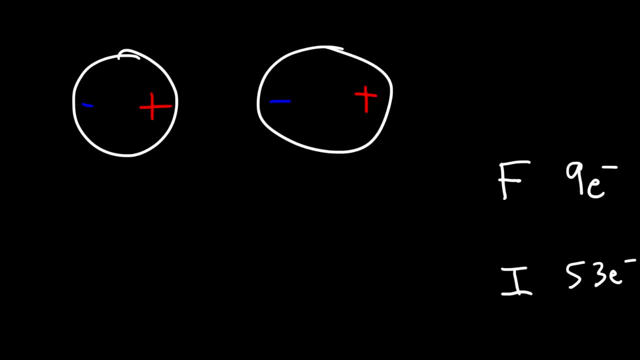 53. So because iodine has a lot more electrons than fluorine, it's more polarizable. It can create a temporary dipole more likely than a fluorine atom. So a temporary dipole will be more likely to form in a nonpolar atom. So a temporary dipole will be more likely to form in a nonpolar atom. 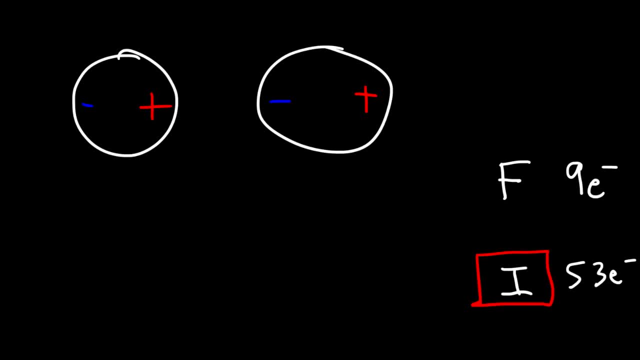 Now notice that the positive side of this atom will be attracted to the negative side of the other one. So these two, they will feel a force of attraction that accelerates them, And so these forces that attracts these atoms together. they're known collectively as: 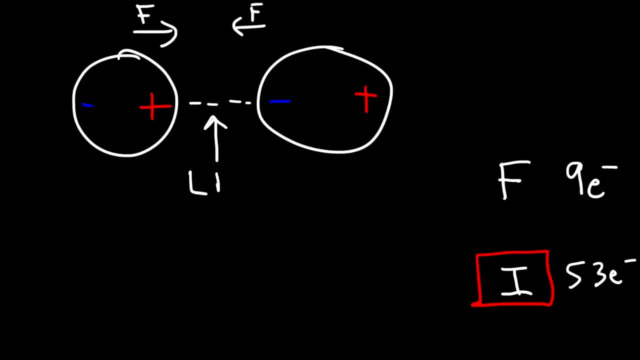 the van der Waal forces, Also known as London dispersion forces. Now this first example. it was a temporary dipole. A dipole is basically a polarized object or polarized molecule, where one side is negative and the other side is positive. 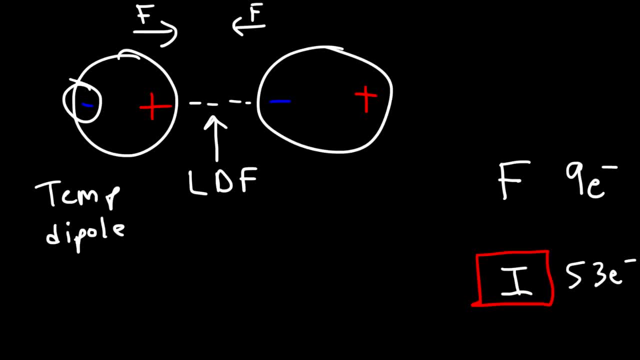 Now, the reason why it's a temporary dipole is because it can go back to its original state. The electrons on the left side can diffuse towards the right side because this negative charge is attracted to the positive charge, And so it can return into its nonpolar state, where the electron cloud is no longer distorted. 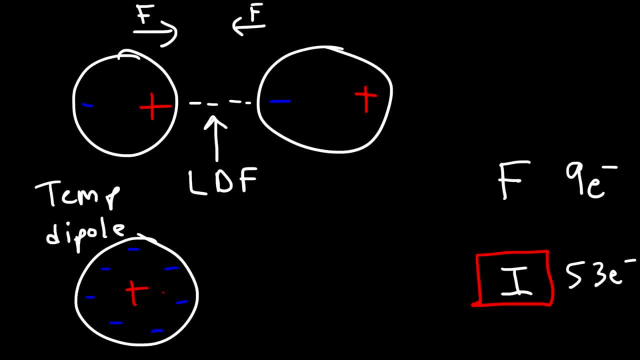 The electrons are distributed evenly, So keep that in mind. This temporary dipole doesn't really last long. It's dependent on the size of the atoms. Now, the dipole on the right is an induced dipole, And the reason why it's called an induced dipole is because it was induced or created. 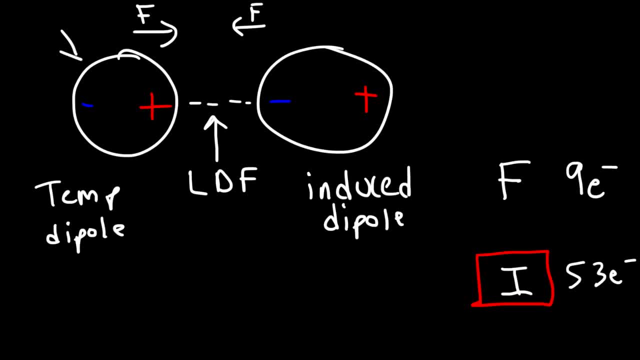 by this first dipole. When this dipole became, when the electron cloud of that dipole became distorted, it caused this, the electron cloud for this atom, to become distorted, thus creating an induced dipole. So make sure you understand the word induced dipole. 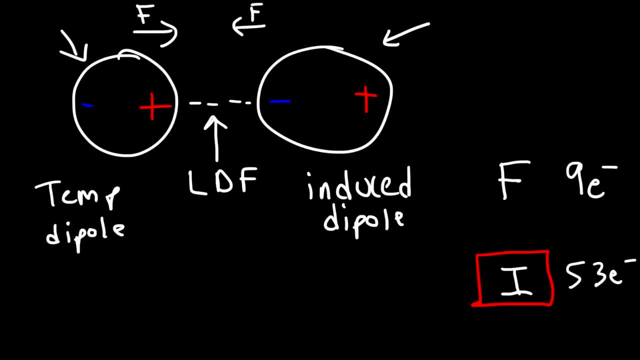 It's just a dipole that was created by something else, So it doesn't last long. It can revert back to its nonpolar state, And so these forces that hold or that attract these dipole-induced dipole molecules together. 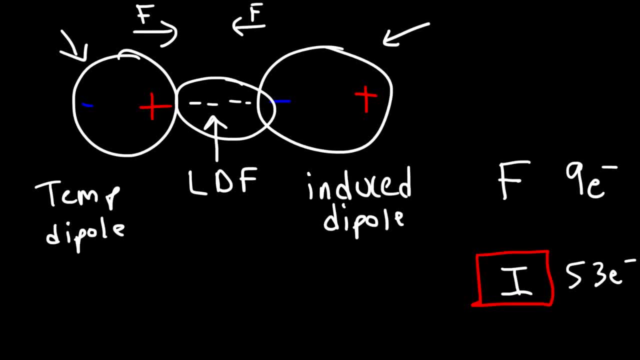 those are the van der Waals forces or the London dispersion forces. They're very weak and they're found in every molecule. However, in nonpolar molecules they are the dominant forces in nonpolar molecules. So these van der Waals forces explain why some nonpolar molecules have higher boiling. 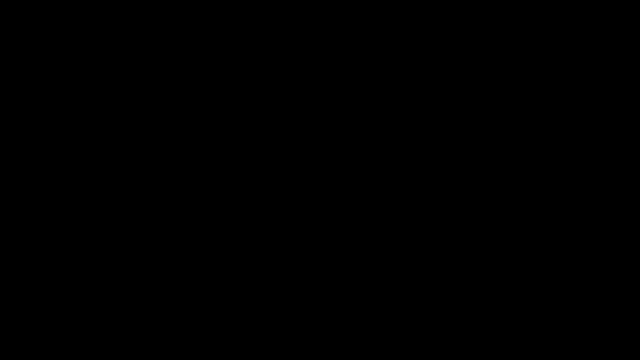 points than other nonpolar molecules. Let's consider the halogens, for example Fluorine, Chlorine, Brine, Bromine And iodine. Fluorine is a gas, Chlorine is a gas. Bromine is a red liquid. 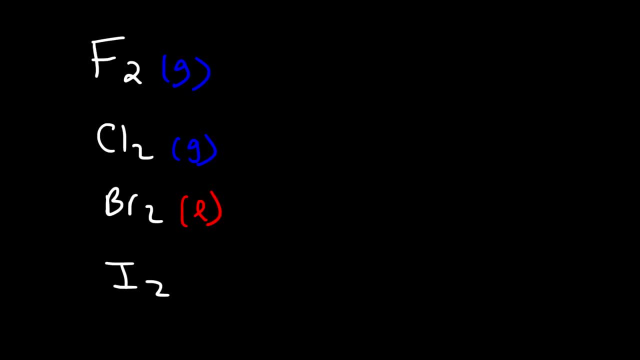 And iodine is basically a purple solid At room temperature, of course. Now, the boiling point of fluorine is negative 188 degrees Celsius, The boiling point of chlorine, it's negative 34 degrees Celsius And for bromine it's 59 degrees Celsius. 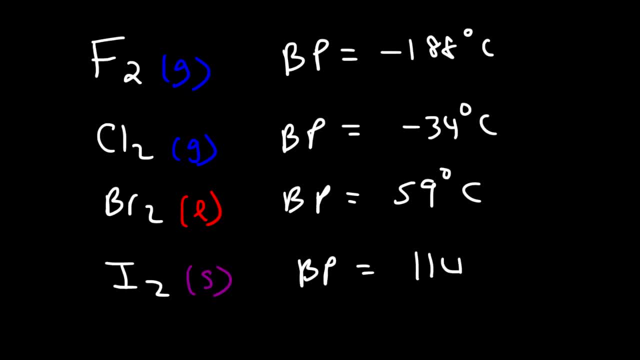 And for iodine it's even higher: It's 114 degrees Celsius. Now if we write down the molecular weight of these molecules, let me get my book out. The molar mass or molecular weight for fluorine is 38.. 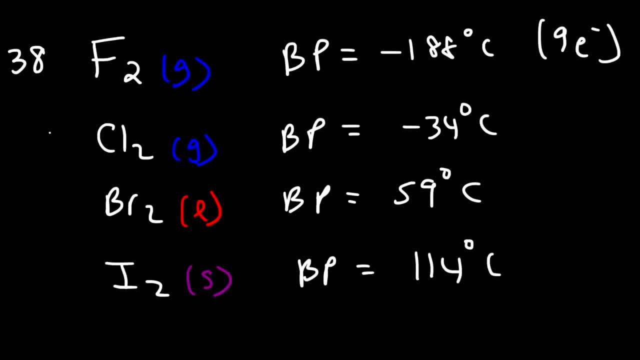 Fluorine has 9 electrons. as we said, The molar mass for chlorine is approximately 70.9.. And chlorine as an atom has 17 electrons. Bromine's molar mass is almost it's like 159.8.. 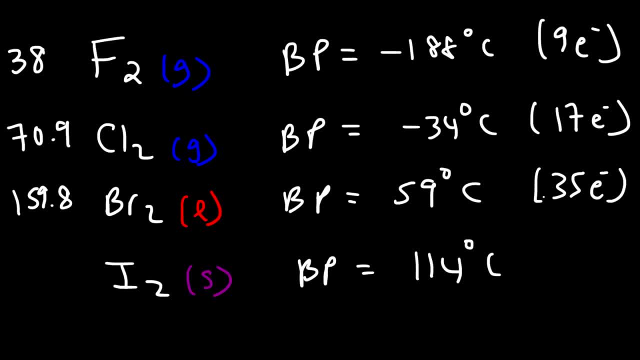 And it has 35 electrons per atom And for iodine we said it had 53 electrons And its molar mass is about 253.8.. So as we travel down the periodic table in group 7a, that is the group where all the halogens are, 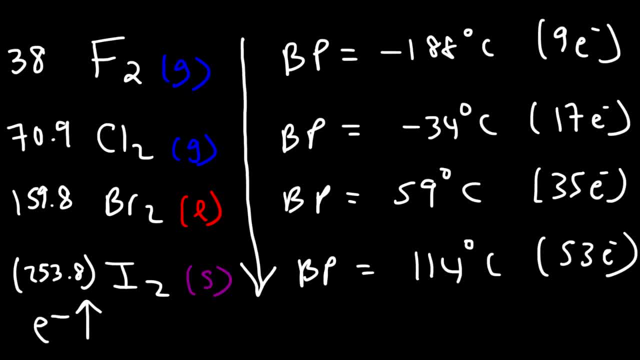 notice that the number of electrons increases, And so the molecules are becoming more polarizable due to the increased number of electrons, And so the molecular weight and the number of electrons. they're proportional, So as a molecule's molecular weight increases. 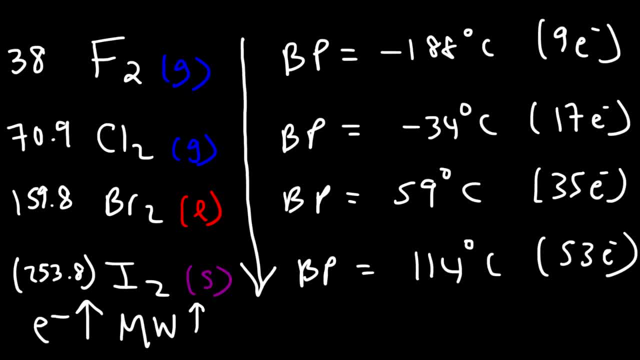 the number of electrons will increase with it too. Now, with molecules that have a high number of electrons or a higher molecular weight, those electrons will- I mean those molecules will- have more London dispersion forces, or more LDF forces. 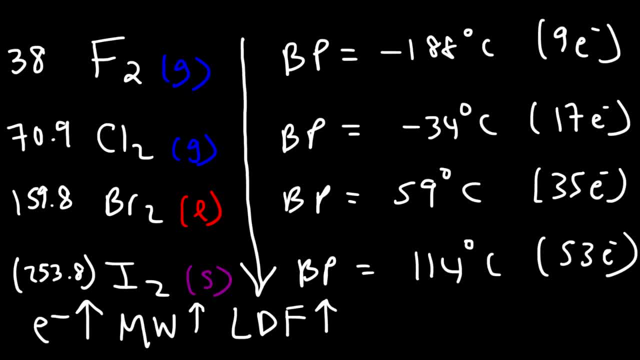 Or you could say Van der Waal forces, they're the same, And so, as that goes up, you could see the trend with the boiling point. The boiling point increases, So iodine has a higher number of electrons. So iodine has a higher number of electrons. 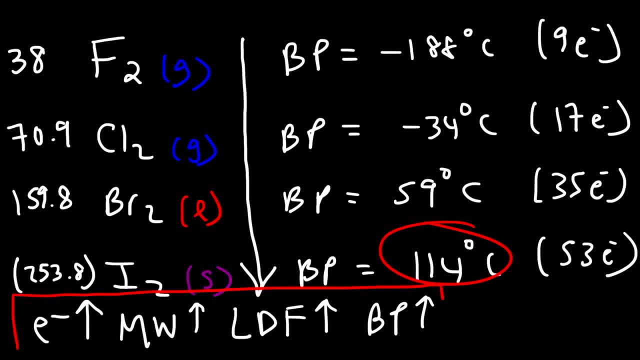 So iodine has a higher number of electrons, So iodine has the highest. So make sure you understand this relationship. So molecules with more electrons or higher molar mass values, they will have more Van der Waal forces. 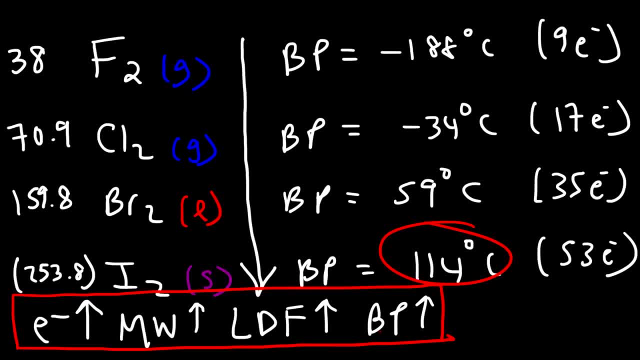 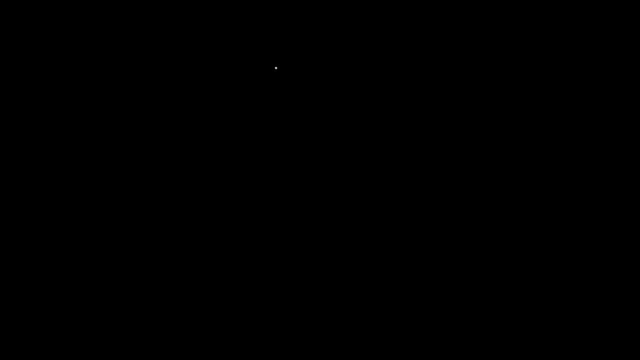 and thus they will have a higher boiling point. So boiling point is directly related to the amount of LDF forces that a molecule has. So here's a question for you. Consider the molecules methane, ethane, propane and butane. 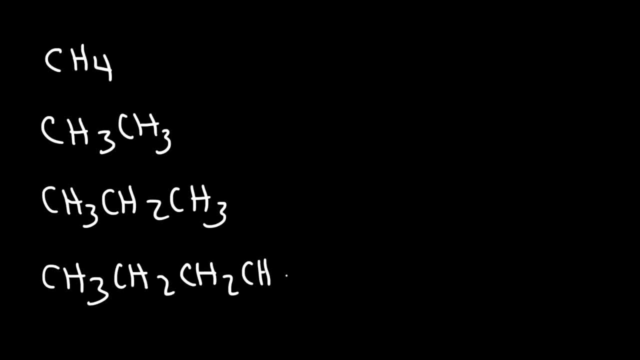 So which of the following four molecules will have the highest boiling point? So, looking at the chemical formula, this is C1H4.. Ethane has two carbons, six hydrogens. Propane has three carbons, eight hydrogens. 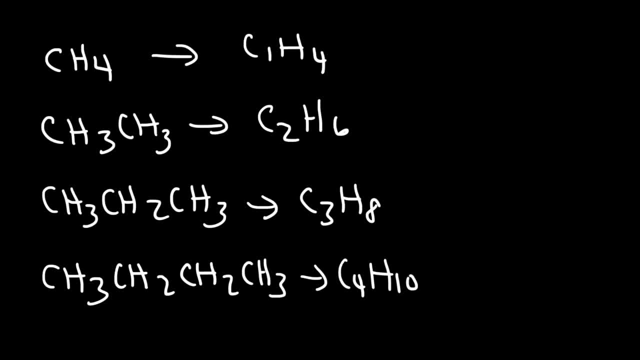 And butane has four carbons and ten hydrogens. So if we analyze the molar mass, analyze the molar mass of each of these molecules, carbon is about 12, hydrogen is 1. So methane has a molar mass of 16.. 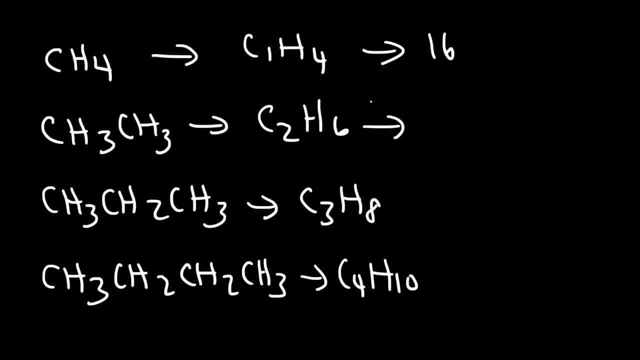 Ethane is going to be 2 times 12,, that's 24, plus 6,, so approximately 30.. 3 times 12 is 36, plus 8, 44.. 4 times 12 is 48, plus 10,, so 58.. So the molecule with the highest molar mass is going to have the highest boiling point, So it's going to have the highest boiling point. So it's going to be butane. Methane has the lowest boiling point because it has the lowest molar mass. 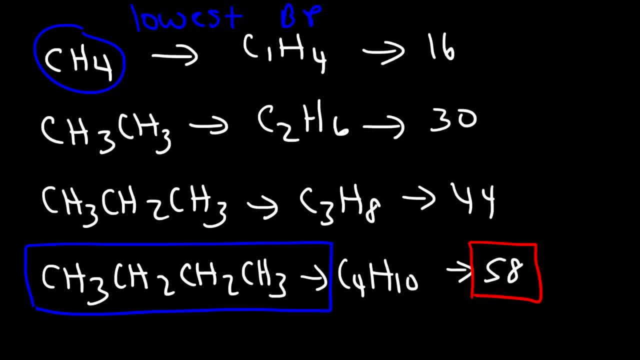 All of these molecules are non-polar. Anytime you have a hydrocarbon that contains only carbon and hydrogen bonds, it's a non-polar molecule. Therefore, the predominant intermolecular force acting on it will be London dispersion forces or Van der Waal forces. 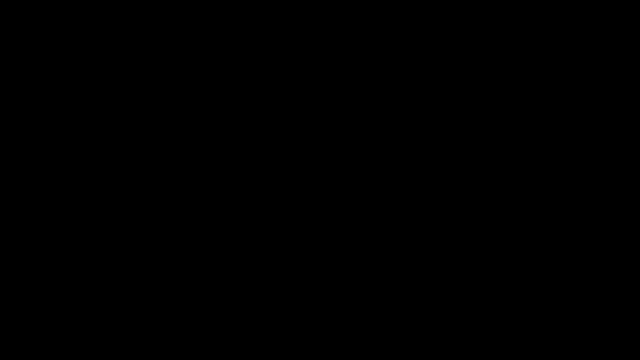 So the most important thing here is to have the lowest boiling point. So we're going to have the lowest boiling point, which is the lowest boiling point in the world, and then the highest boiling point is the lowest boiling point. The lowest boiling point is the highest boiling point in the world. 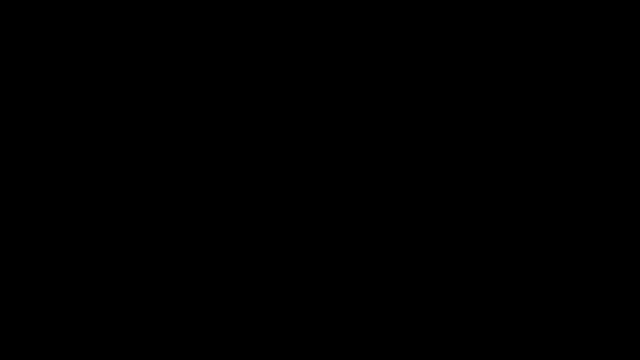 So you can see how the number of molecules is going to change. So it's going to be about 11..